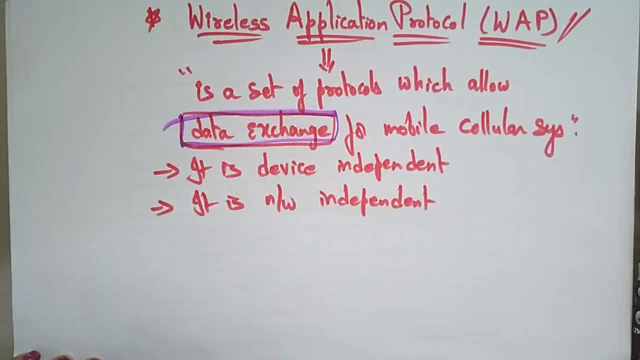 exchange for mobile computing, data exchange for mobile computing. But so it is a device independent as well as a network independent. Okay, so I want to just give a brief. like the current constraints of wireless interface and the mobile devices so far you are using, 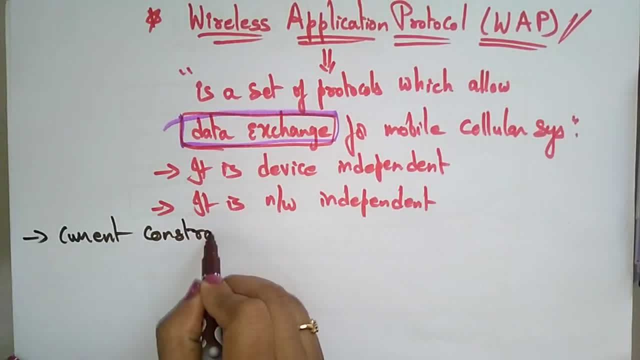 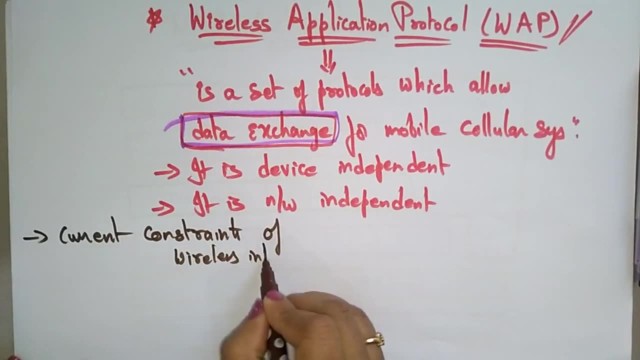 Current constraints of, let's take the wireless interface. So, whatever the wireless interface you are taking, and the mobile devices. So what are the current constraints of these devices So which are not using the WAP? So here are the current constraints for this is the wireless interface, is 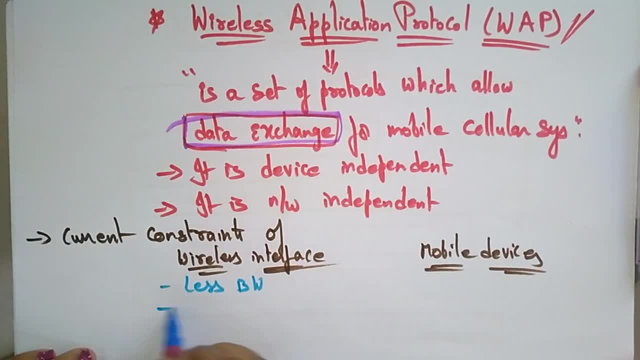 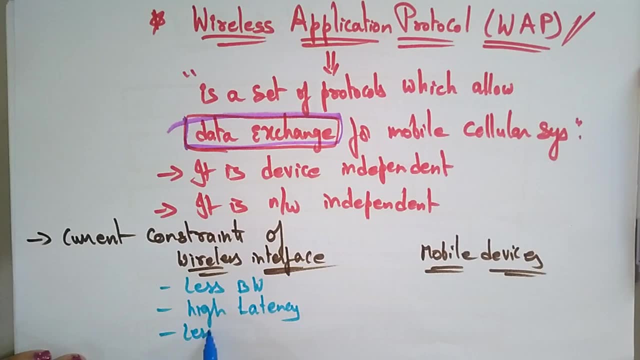 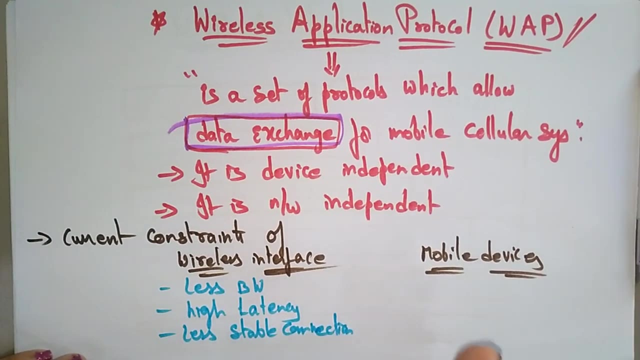 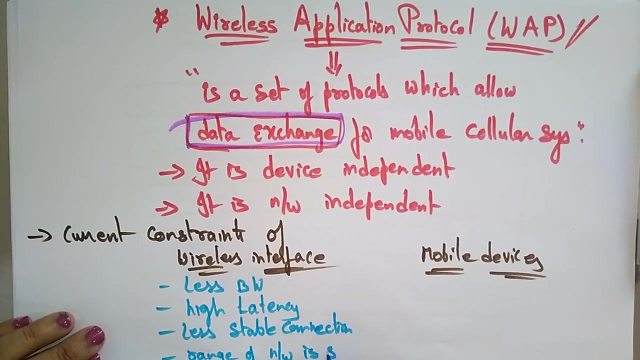 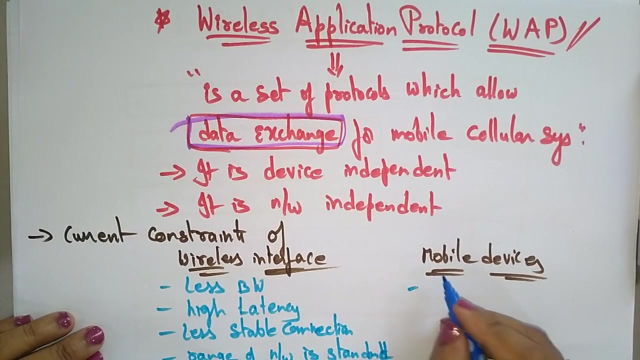 having the less bandwidth and it's having the high latency and less stable connection. The device range of network is standard. The range of network is. device range of network is standard. these are the constraints for the wireless interface. then, whatever the mobile devices constraints, it is here the mobile devices: less CPU power and less. 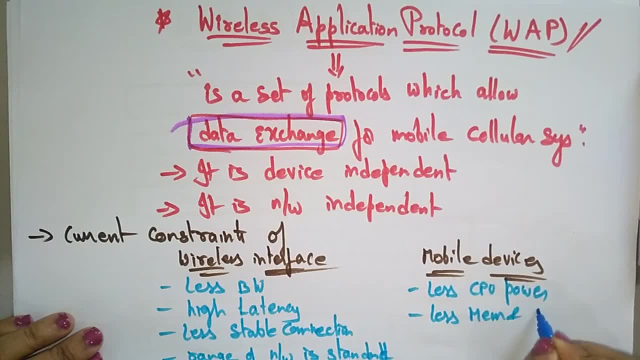 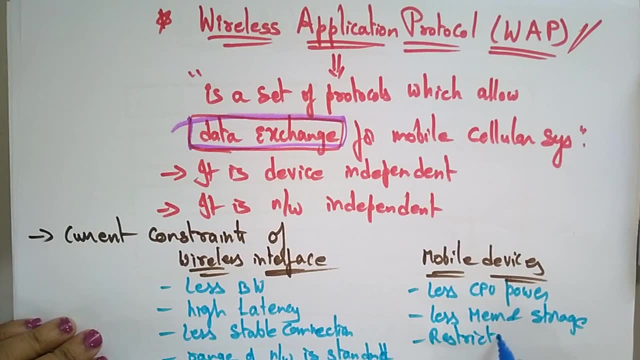 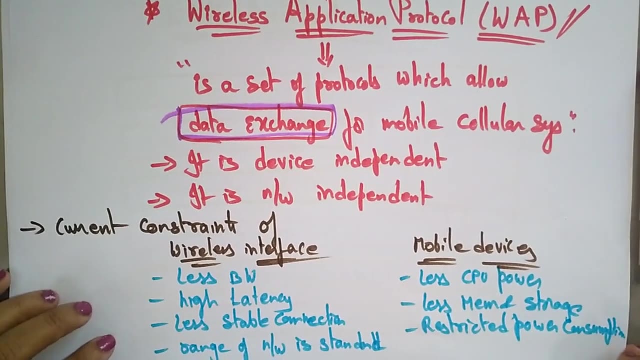 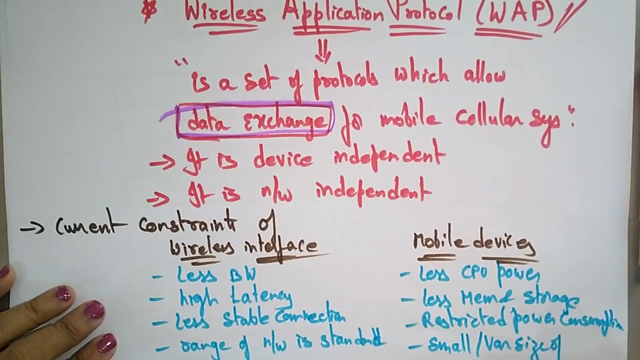 memory and the storage. less memory and storage. restricted power consumption. restricted power consumption and a small or variable size of fur displaces small or variable size of display. so these are the current constraints of the, a device which we are going to discuss in the next class. 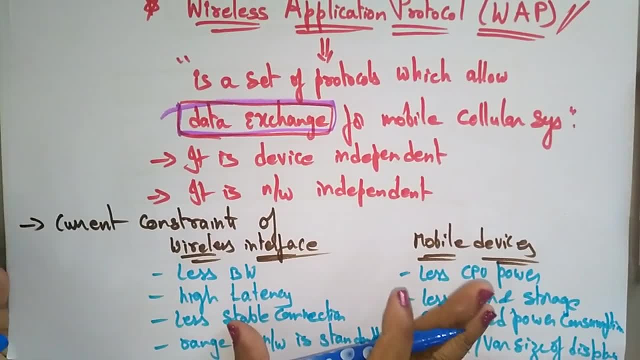 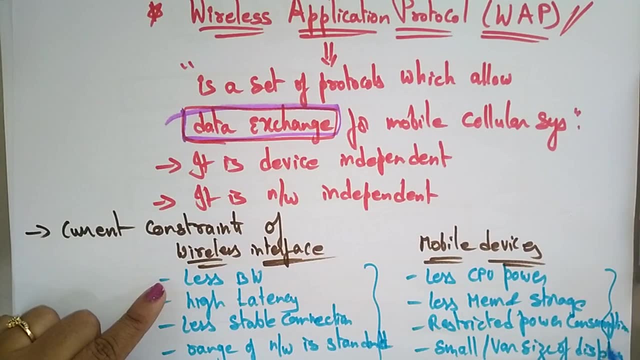 whether it any wireless interface or the mobile devices. so, even though these these having these type of constraint, the wireless interface is having these constraints and the mobile device are having these constraints, even though it's having a drawbacks, the wireless application protocol is supporting these wireless interface as well as the mobile devices, because it is a 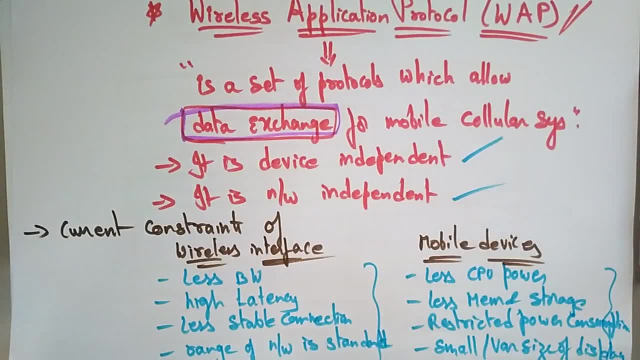 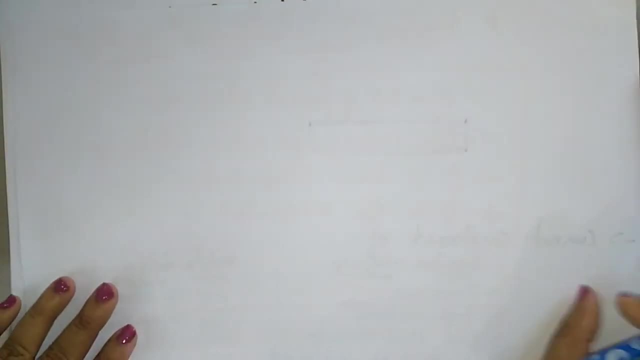 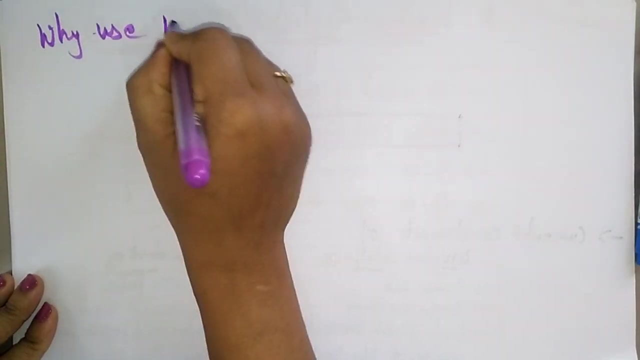 device independent and the network independent, so it doesn't bother about what type of device using and what type of network you are using. the wireless application protocol is a is set of protocol which allows the data exchange for mobile cellular system. ok, now let me explain you why we use WAP, why use wireless application protocol. 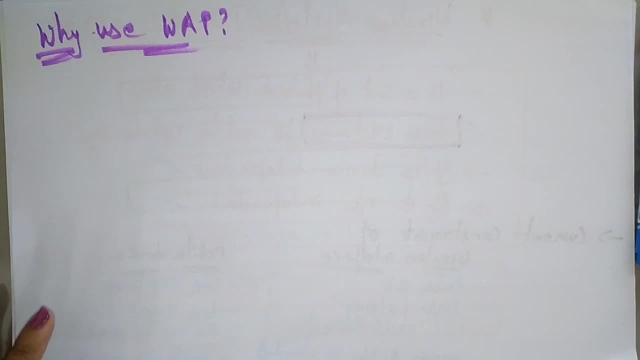 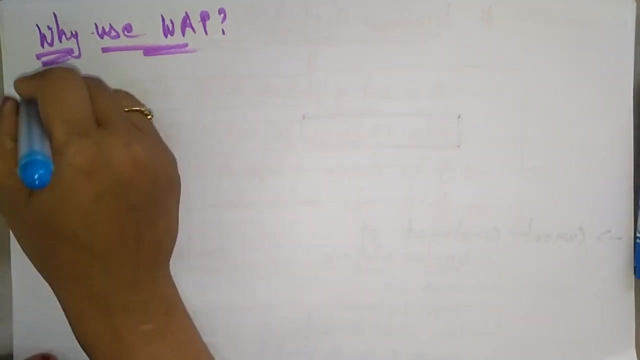 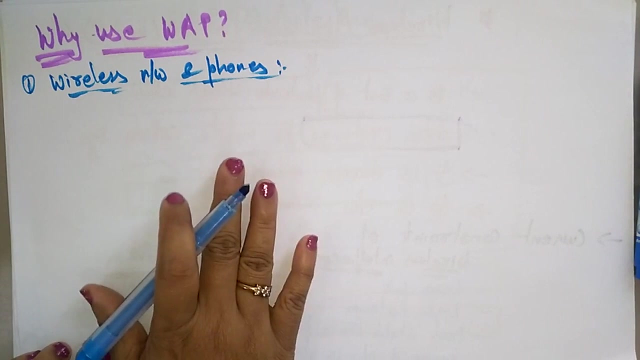 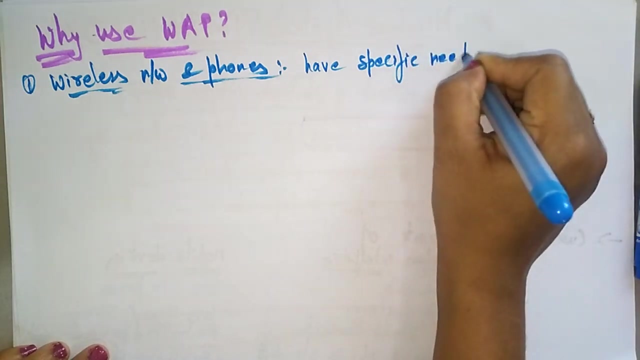 so what is the need of using this WAP wireless application protocol? actually, the wireless network and the phones, yes, So if you take the wireless network and mobile phones, if you take. So let me explain why we are using VAP here. If you take the wireless network and the phones, which have a specific needs and requirements. 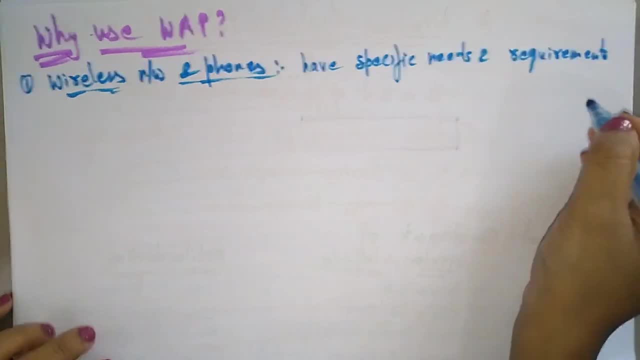 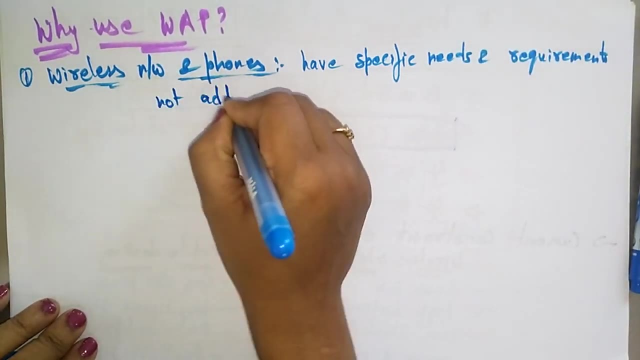 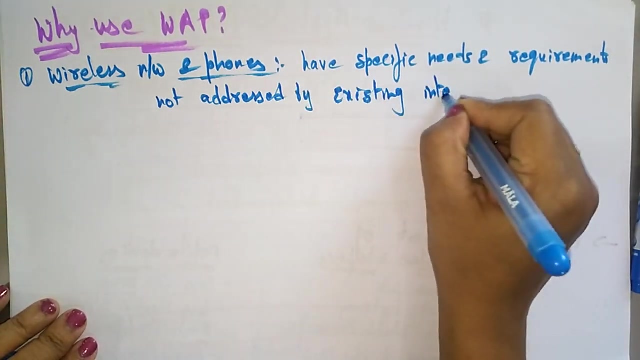 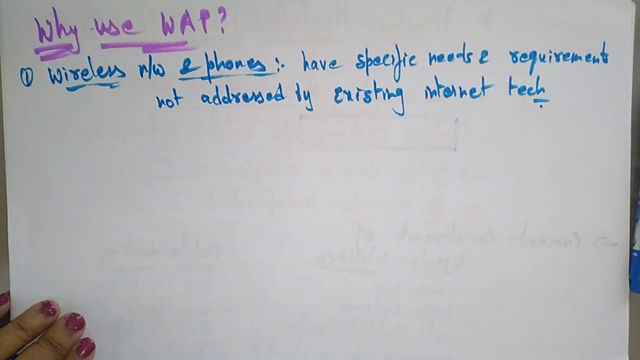 So the wireless networks and the mobile phones have the specific needs and the requirements not addressed by not addressed by existing internet technology. Actually, wireless networks and the phones is having the specific needs and the requirements but which are not addressed by the existing internet technology. So, if it is not addressed by the internet technology, 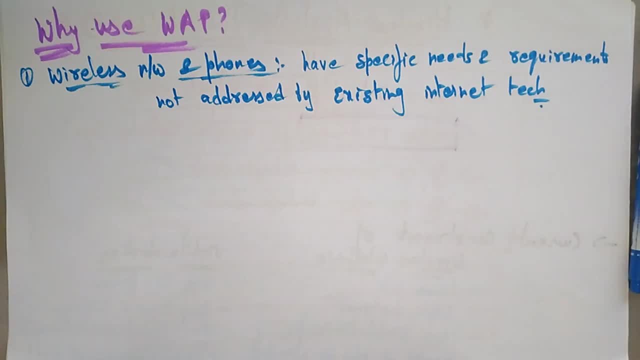 Some protocols will not support. but VAP is a device independent and the network independent. So it supports for transferring the data between the wireless net, between any systems in the, in the case of wireless networks, or it may be a phone, and next a VAP enables any data transport. VAP enables any data. 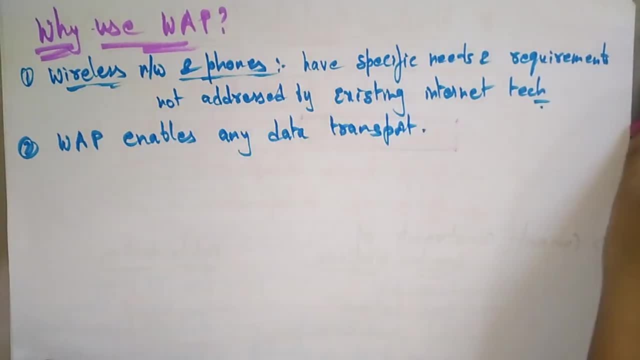 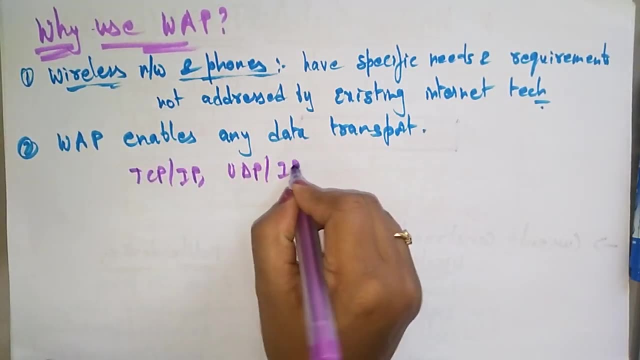 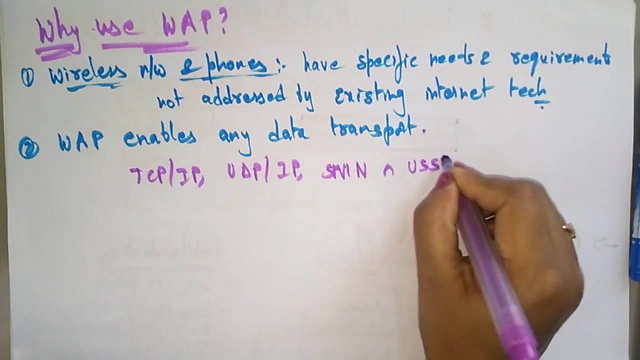 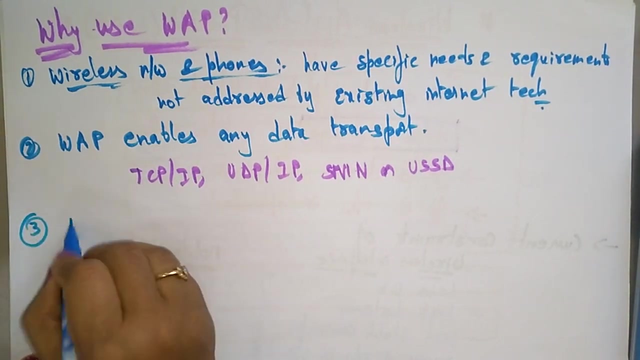 iez it via it to What the adapters can you get? is this r? So if you right, then you can enter theester and you go through it In this, in this document, you can enter each Formation, okay, And in theíre server we do not need R.